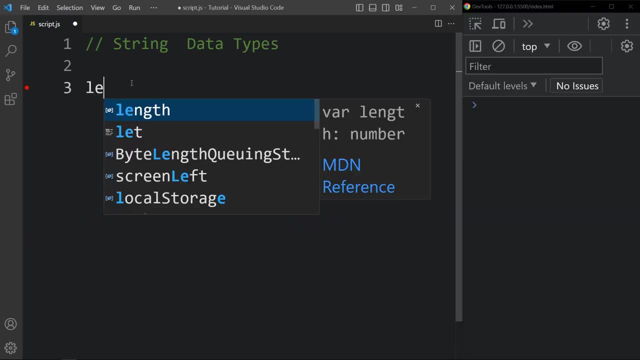 and manipulating text. For example, If I write Let firstName equal to double quote Elon. So here we are adding one name in double quote. It is a string and the variable name is firstName. Let me duplicate it. Here we will add lastName. 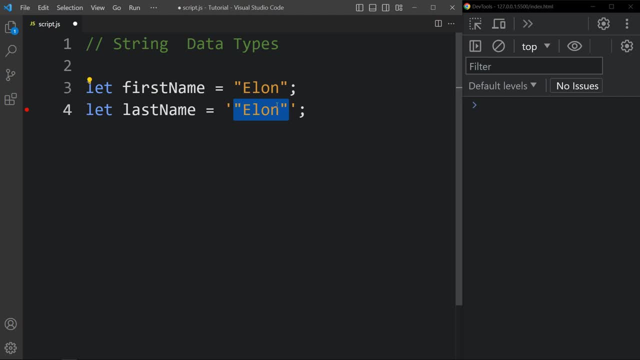 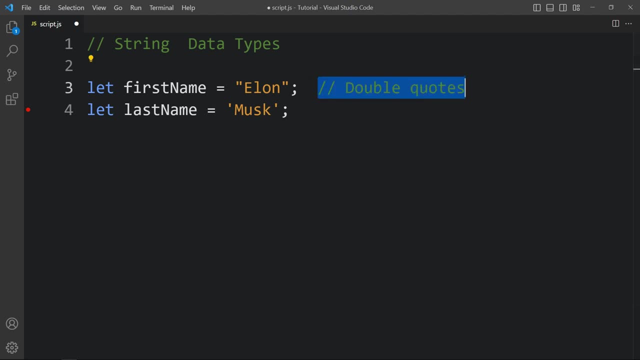 And if I write the text in single quote, Musk, It is also a string, It is written in double quote And this is written in the single quote. Now let's see another data type, which is number. Number represents integer and floating. 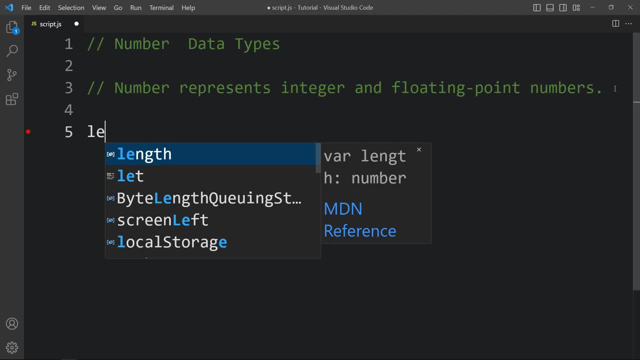 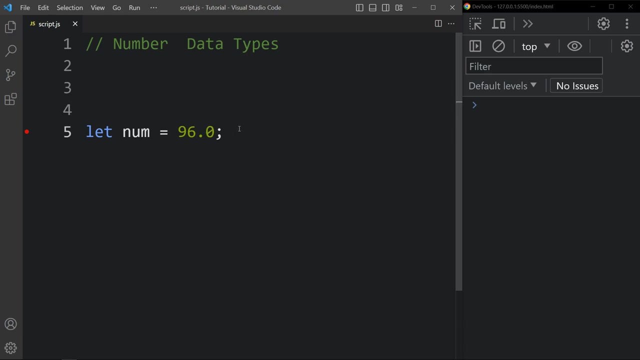 point numbers. For example, if I write let num equal to 100. In this statement we have declared one variable called num and initialized its value with the integer 100. let me change the value. if i write 96.5, it is also a number type. here we have stored the floating number. if we write 96.0, then javascript. 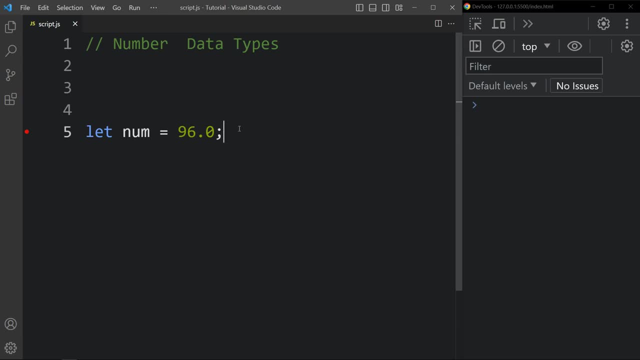 will convert it into an integer number to use less memory, so it will be saved only 96. let me show you that if i write consolelog num so you can see 96 is printed here, it is not printing 96.0, it is printing 96 only because the javascript is converting this floating number into an integer. 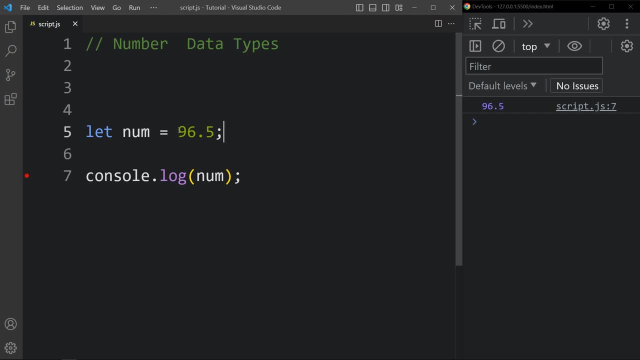 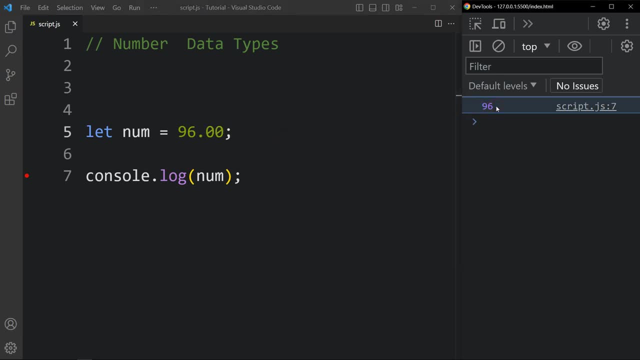 96.5, it will be saved as 96.5, and if we change 96.5, it will be saved as 96.5, and if we change 96.0, it will be only 96. now let me take another example. if i write, let x equal to 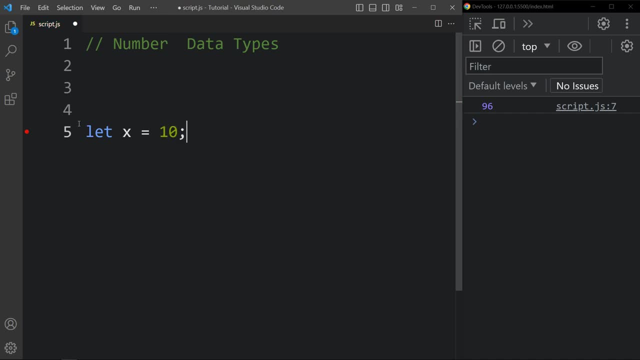 10. so here i have a stored one number in the x variable. let me write consolelog x here we will get 10 in this console tab. we got 10. Now if I add a single quote in this 10, now it will become string, because we are adding. 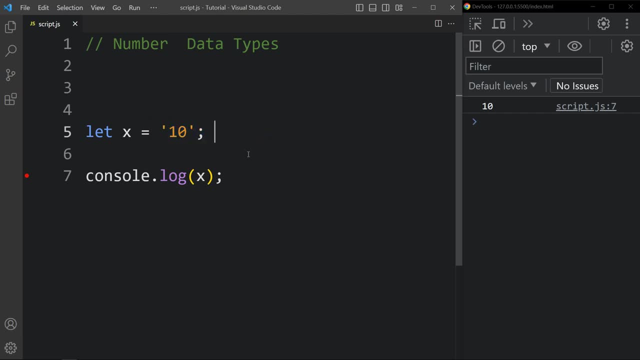 single quote in this text. Now, if I print this one, you can see still it is displaying 10.. But if you will check the data type it will be a string. The value is 10, but the data type is string. To check the data type we have one operator called typeof. 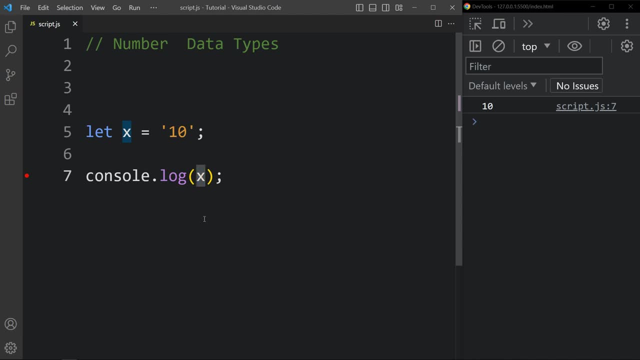 In front of this variable name. if I write typeof, You can see we got the data type string because this 10 is written inside this single quote. If I change it and make double quote, still it will be string. You can see string here. 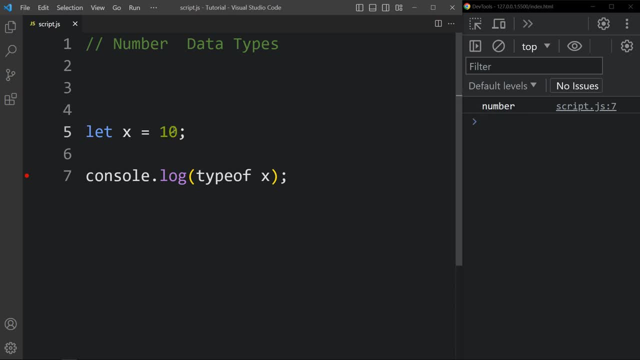 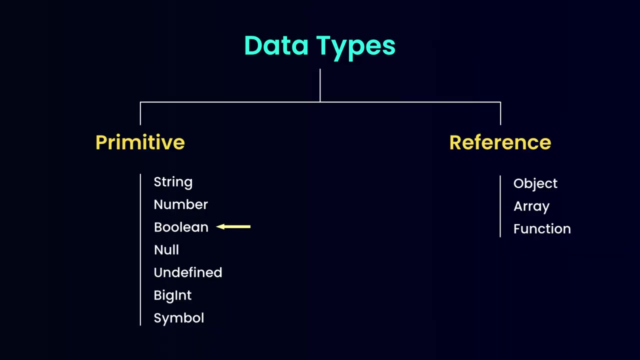 Now, if I remove this quote And if we only write 10, then it will be a number. You can see it is number. When we will add double quote or single quote, it will be stored as a string. Now the next data type is boolean. 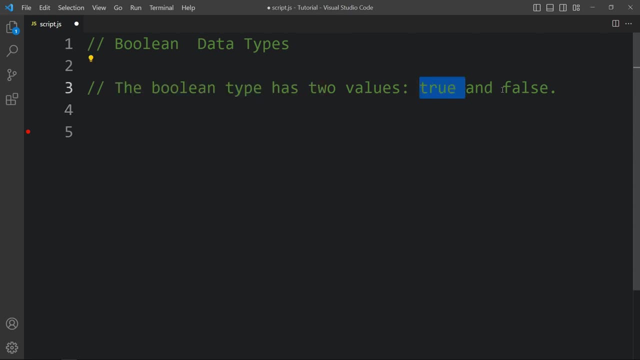 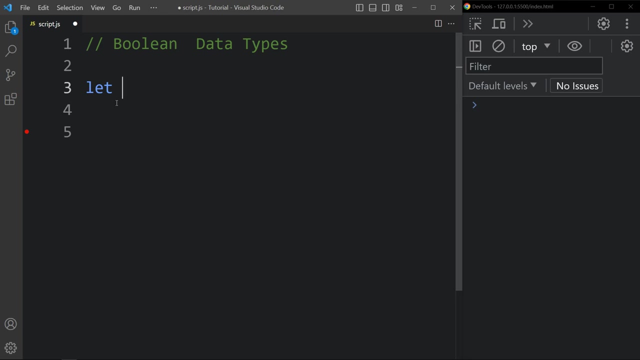 The boolean data type has two values: true and false. Let's understand it with one example. If I write let Learning equal to true And let completed equal to false, Here we have stored boolean data in the learning variable and completed variable. 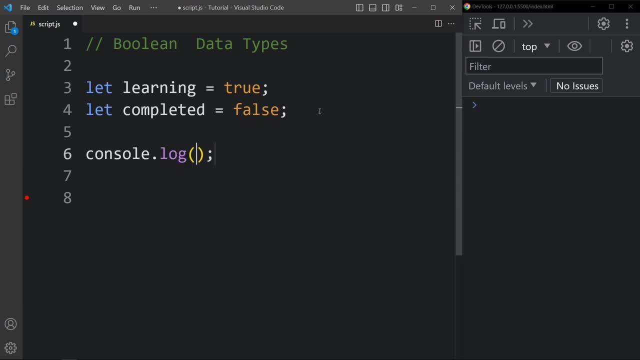 Now to check this one, we will add consolelog learning: false. You can see true, So it is displaying the value stored in this learning. Now to check the type of the data stored in this learning, we will again use the typeof operator. 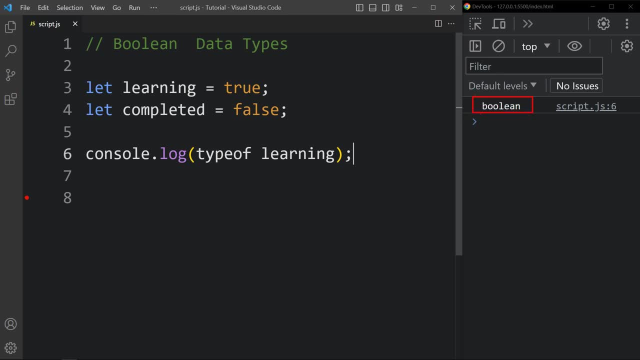 Typeof learning. So it is displaying the data type boolean. Now let's check the data type of this Another variable which is completed. Just copy this one, Add it here Here it will display the data type boolean for the another variable called completed. 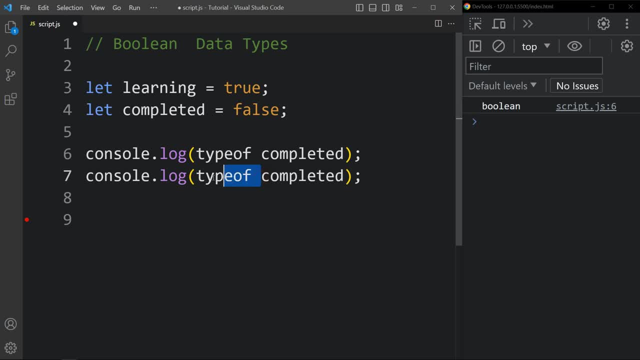 Now, if you want to display the value stored in this completed Here I am adding consolelog completed and it is displaying false here, which is the value stored in the completed variable and it is the type of the value which is boolean. So we have stored the true. 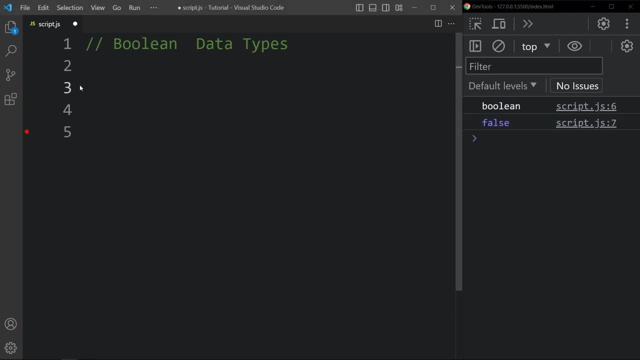 So we have stored the true or false value directly, but we can store the result of any expression. For example, if I write let x equal to 20 greater than 10.. So the result of this is true: 20 is greater than 10.. 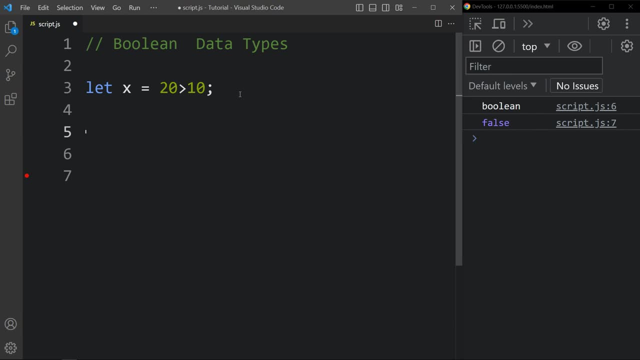 It is true. So now, if you want to check the value stored in the x, We will add consolelog x And now you can see it is displaying true. Here we are writing 20 greater than 10, but the x has stored the result of this expression. 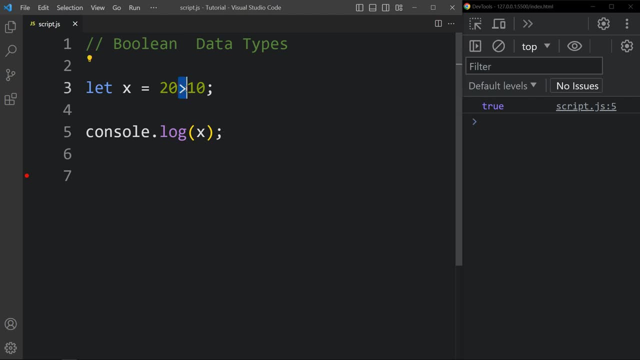 which is true. Now, if I change, If I write 20 less than 10, which is false- So you can see the result in the console tab- It is displaying false. So we have stored the false in the x variable. Now let me show you the type of the data. 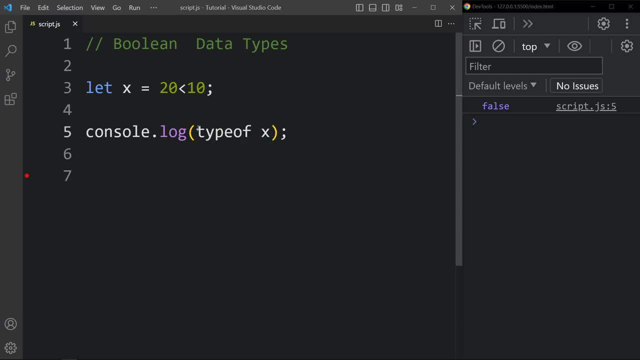 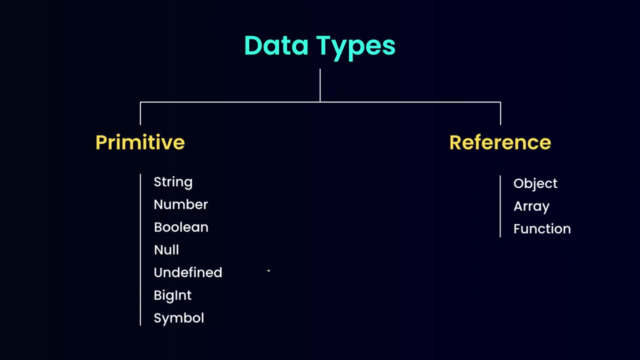 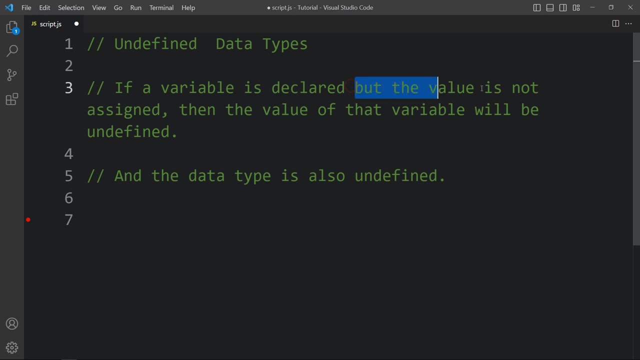 Here we will add typeof x, and now it is displaying boolean. So this x has stored the boolean data type. Next, primitive data type is undefined. If a variable is declared but the value is not assigned, then the value of that variable will be undefined and the data type is also undefined. 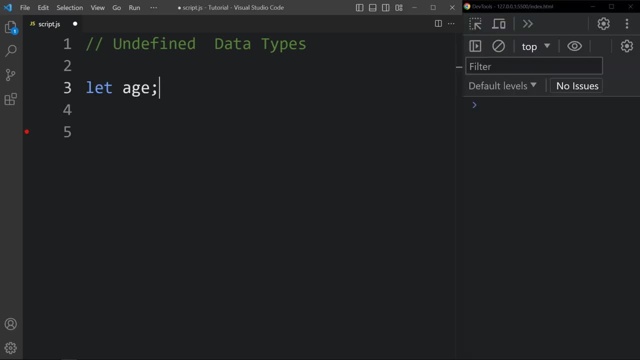 Let me show you this with one example. Let h: We have declared a variable h, but we have not assigned any value. Now we will check the value stored in this h. Let's add consolelog h Here you can see: the value is undefined. 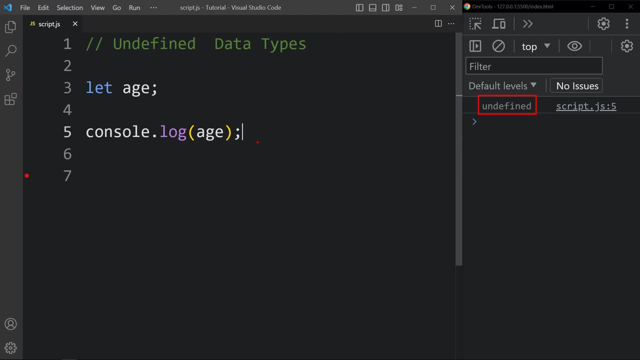 Now, if you want to check the type of the data, Here we will add consolelog typeof age. Now you can see the value is also undefined and the type is also undefined. If we add any value like this: age 30. Now you can see the value is 30 and the type is number. 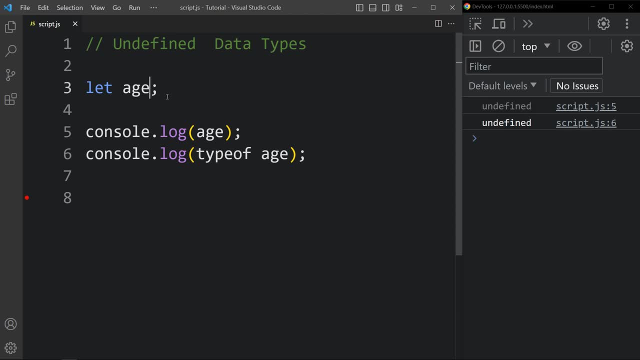 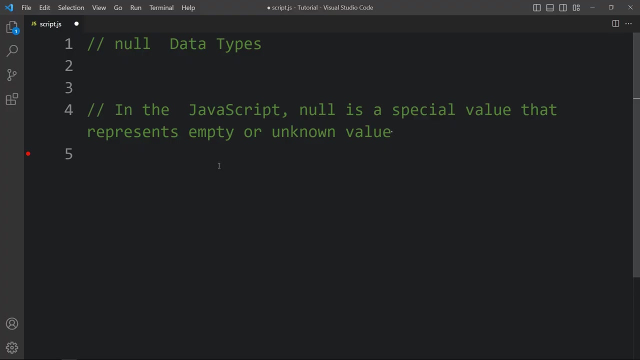 And when we remove it We have got the value. We have not assigned any value, So the value is undefined and type is undefined. So this was undefined. data type: Next, primitive data type is null. In the javascript, null is a special data type that represents empty or unknown value. 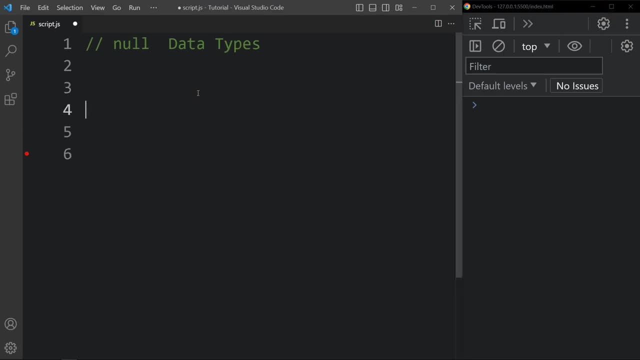 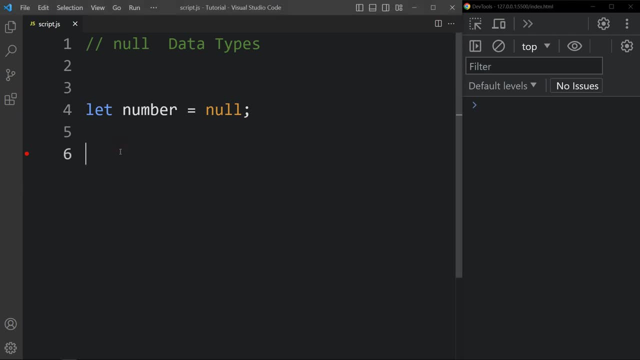 Let number equal to null. And now we will try to print the value. Here we will add consolelog number, So you can see the result. It is displaying null. Now we will try to display the type of the data. So here in the next line we will add consolelog typeof. 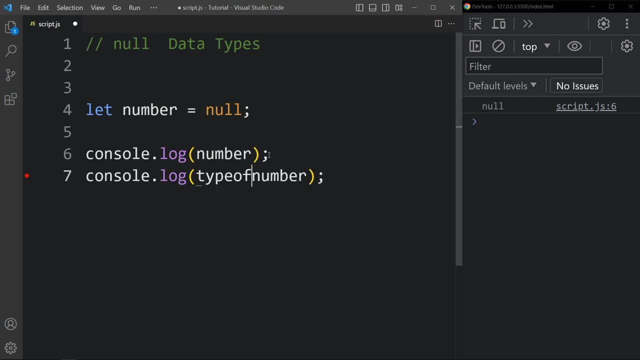 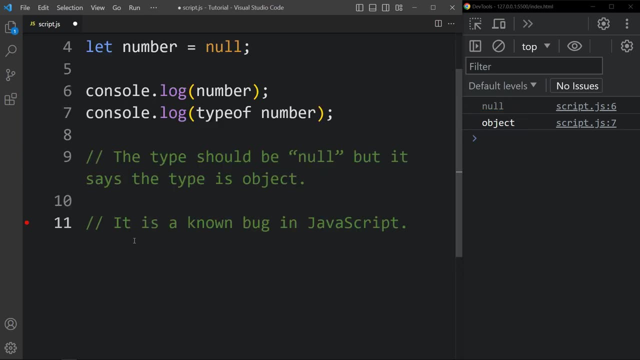 type of number. you can see the value is null, but the type is object. the type should be null, but it says the type is object. it is a known bug in javascript. javascript defines that null is equal to undefined. to check this one, we will write consolelog. 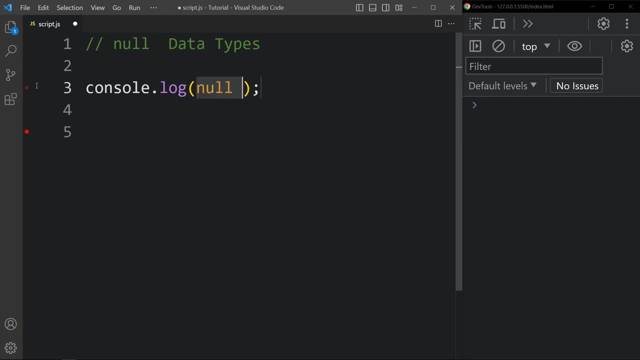 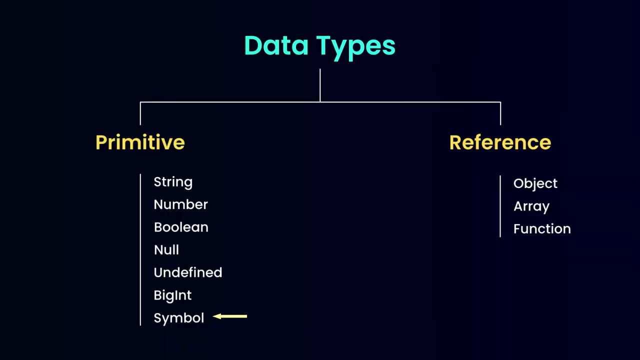 null comparison operator, then undefined. so we are comparing null with the undefined and here you can see we got the result true, it means in javascript, null is equal to undefined. there are two other primitive data types which are symbol and begin. that we will study in our upcoming videos. 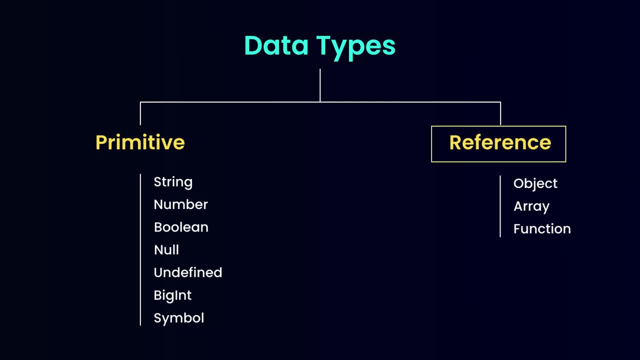 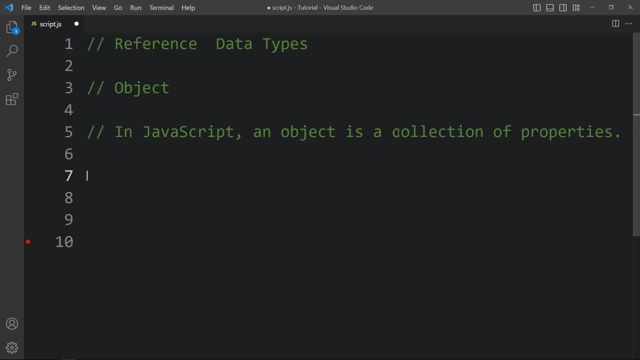 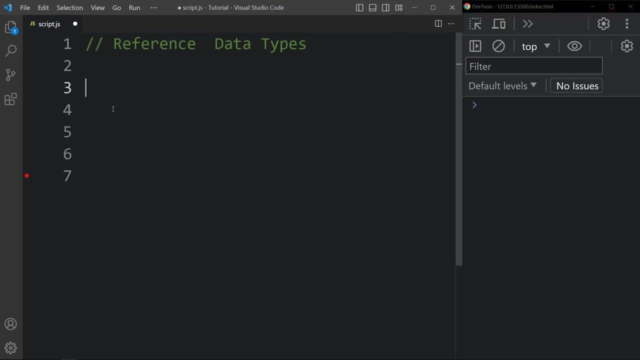 now let's learn about the reference data type. so the first reference data type is object. in javascript, an object is a collection of properties where each property is defined as a key value pair. so let me create one object here. if i write let person equal to curly braces, that's it. so the following code defines an empty object. this is the person. 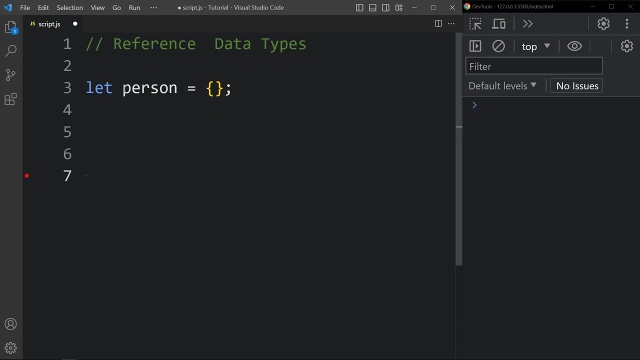 object which is empty. now let me display the data stored in this person object. for that we will add consolelog person. that's it now. you can see we got the empty curly braces. now to check the type of the data, we will copy this one and here we will add type of person. so you can see the 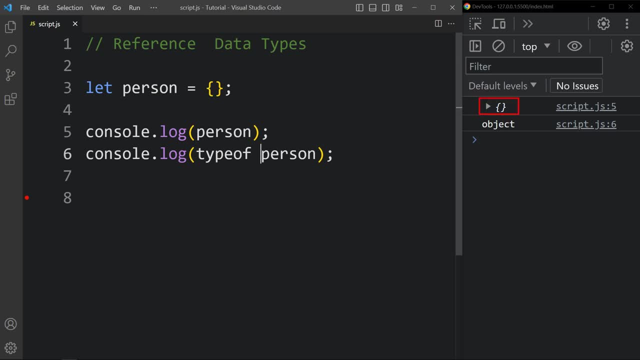 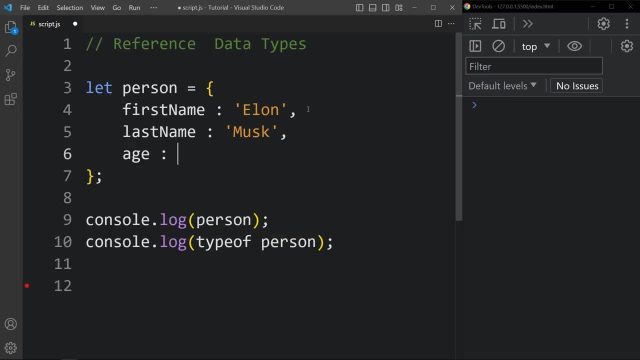 and age. let's add 35, so you can see in the console tab the data type is object and this is the data stored in the person object: first name: elon. last name: musk. age 35. an object can store different data type in this person object: the first name and the last name. 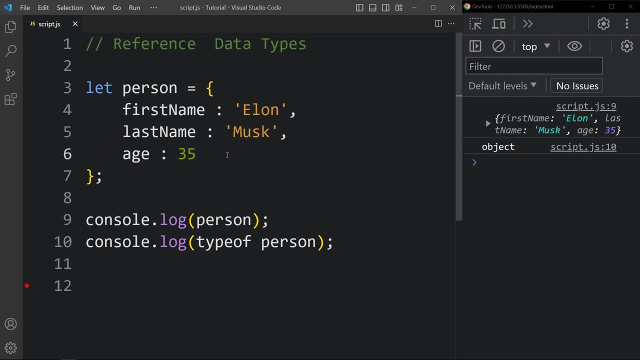 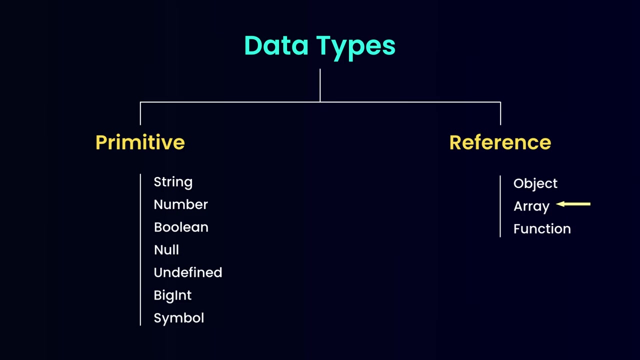 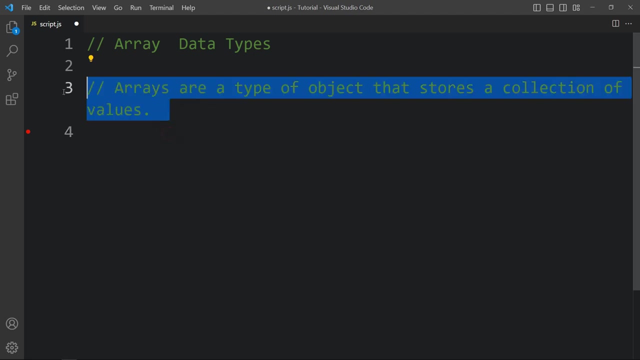 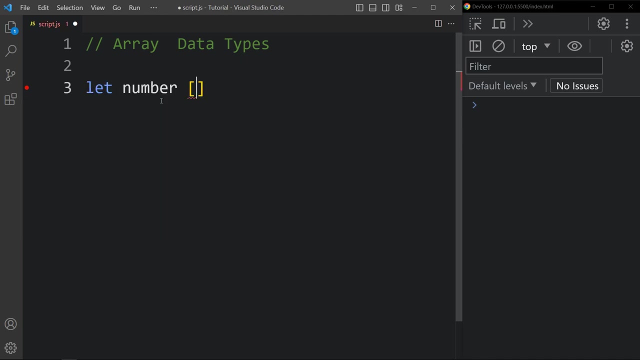 are string and this age is number. so this person object can store different type of data. it can also store another object. our next reference data type is array. arrays are a type of object that stores a collection of values. for example, if i write let number, we have added five different number separated by comma in the square bracket. so the following: 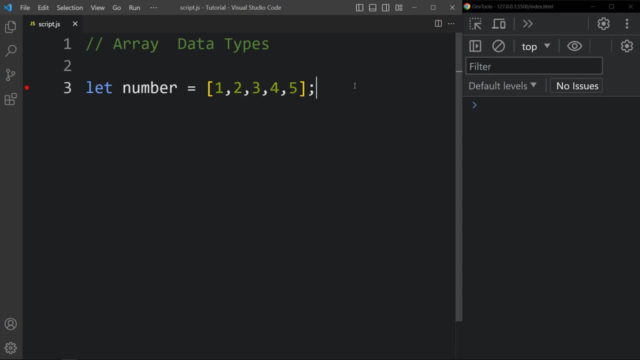 code creates an array of numbers. now let's print the value of this number. we will add consolelog number. so in the console tab you can see this array is printed: 1, 2, 3, 4 and 5. the same thing is printed here. now, if you want to check the type. so let's add this line again and in this: 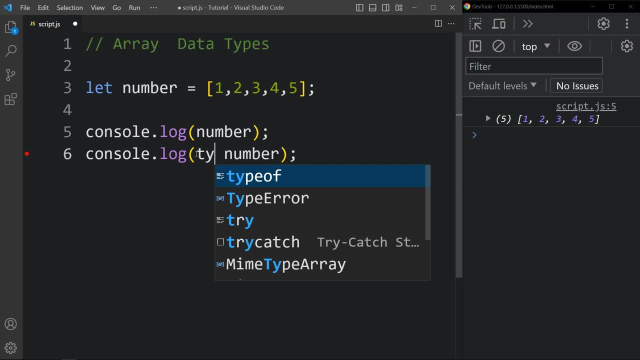 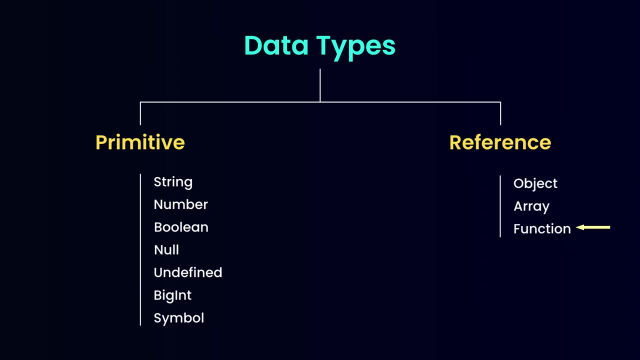 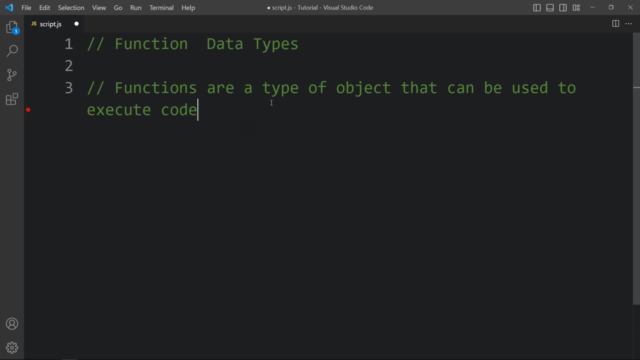 one we will add type of operator, type of number. now you can see in the console tab we got the type object, so the array is also an object data type. our next data types is function. functions are a type of object that can be used to execute code, for example. here we will create: 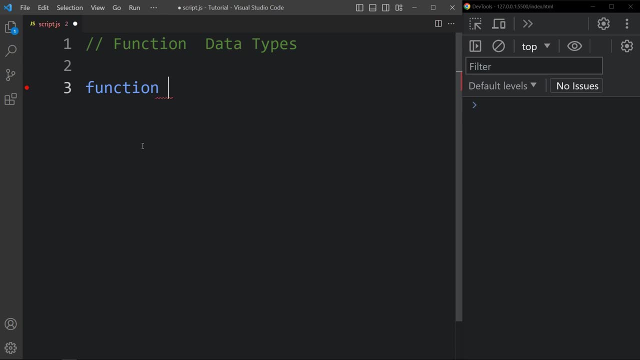 one function. to create a function, we use the function keyword and the name of the function. so we'll add in the message string and another one among the function name, msg. i also made a memory V Forest, so let's add the function name msg. that is for the message and in this. 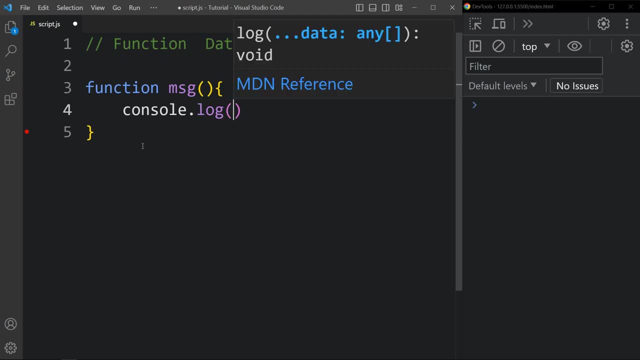 one. just add one consolelog and here we will add one string: hello, greatest stack. so we function name: msg. now if you want to check the type of the data here we will add consolelog type of msg. that is function name. and if i check this in the console tab you can see: 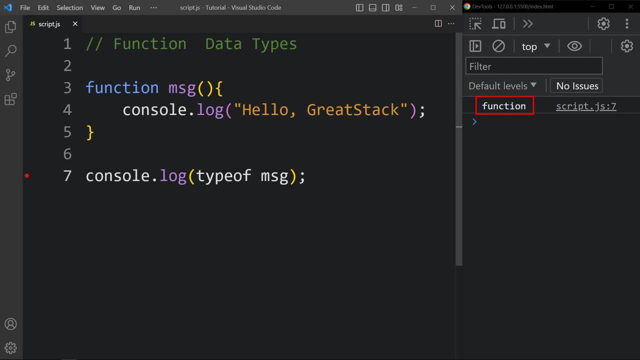 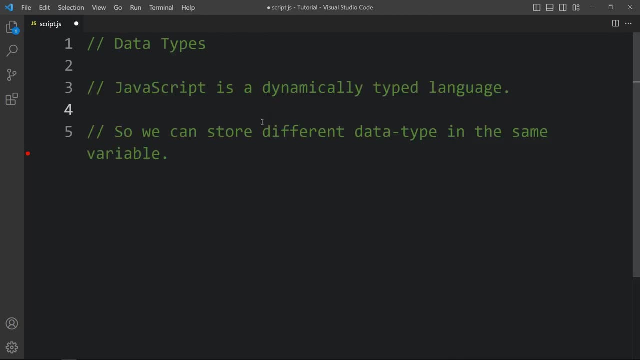 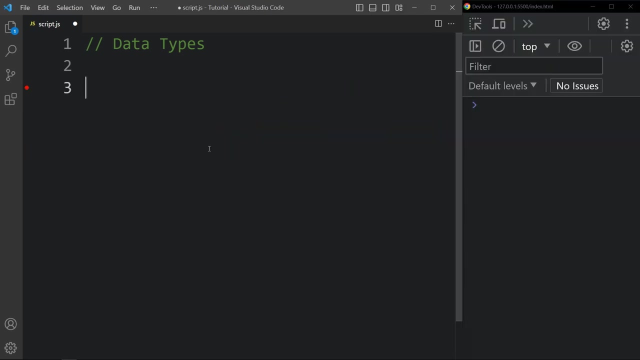 it is displaying function. it says the type of data is function, but it is also an object data type. javascript is a dynamically typed language so we can store different data type in the same variable. for example, if i write let x here, we are not assigning any value, so the data type will be. 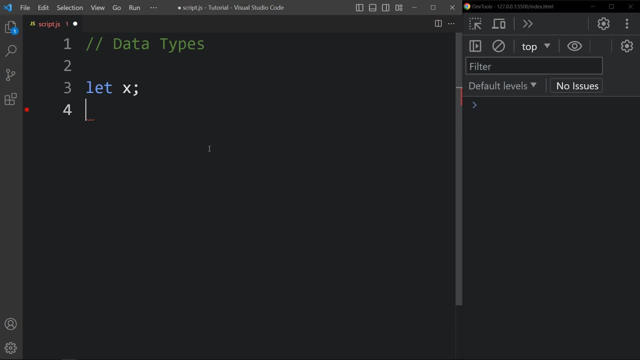 undefined. so let's check this one type of x. it is displaying undefined. let's check the value also. if i write consolelog x, consolelog type of x, so it will display the value stored in the x and it will display the data type. now you can see in the console tab it is displaying the value undefined. 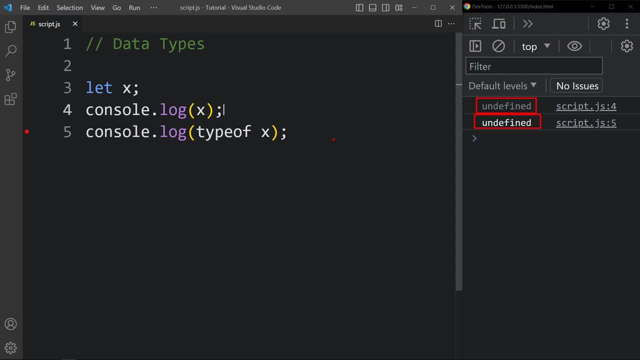 and data type undefined. now in the same variable we can store different data type. here we have already declared the variable, so we will just add x. we are not declaring, we are just assigning the value x equal to, let's say, one string greater stack. so here we are adding one string in the x variable. let's try to print this: 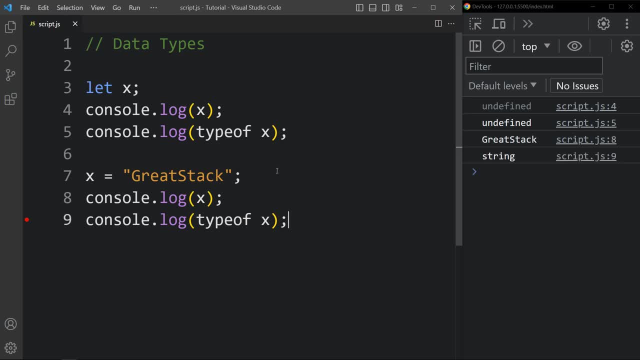 you can see in the console tab, it is printing undefined and undefined from here. now we have changed the data. it is greater stack, which is a string. so you can see the value and the data type is a string. now again, we can change the type of the data. we will simply store another data. 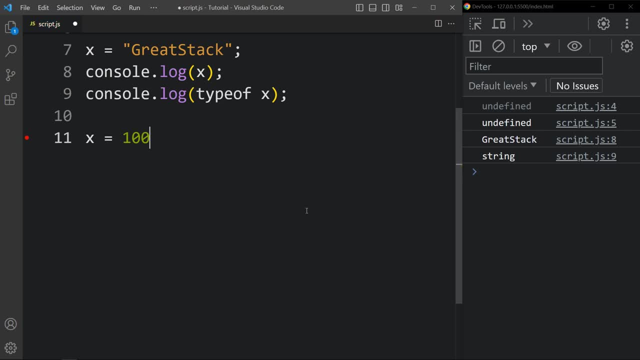 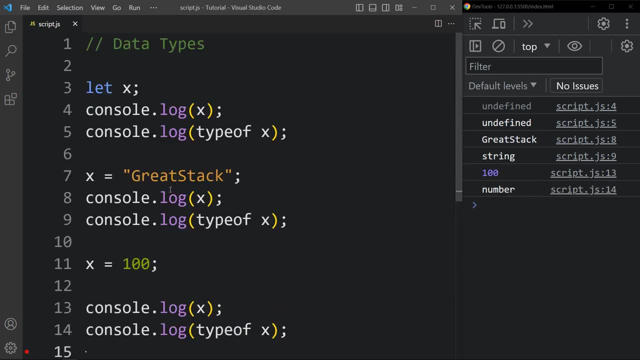 let's add x equal to 100. so here we have stored the number. let's try to print this now. you can see in the console tab we have the value 100 and we have the type number. so earlier it was undefined. then it is a string.